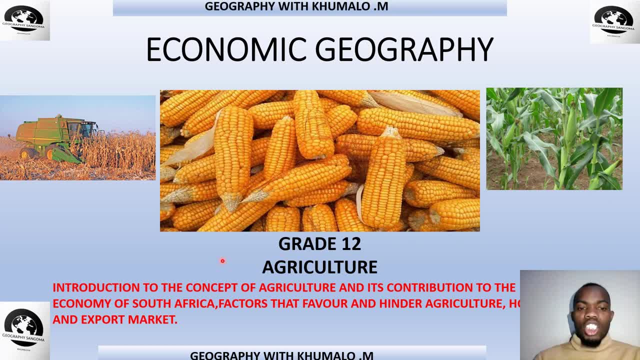 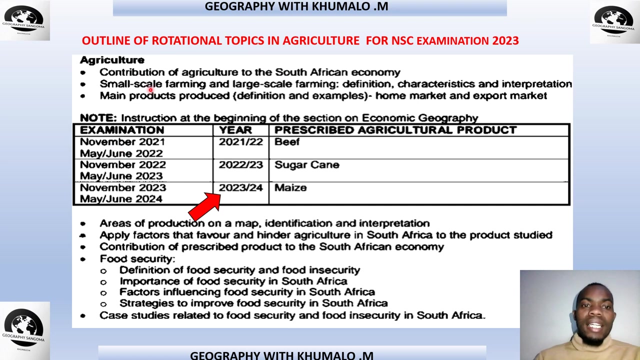 Now today we are going to look at the introduction to the concept of agriculture and its contribution to the economy of South Africa, factors that favor and hinder agriculture, and also look at the concept of home and export market. Now Grade 12s. I want to outline something here that is from your exam guideline. Now in agriculture we've got rotational topics. It means that we deal with a certain agricultural problem. 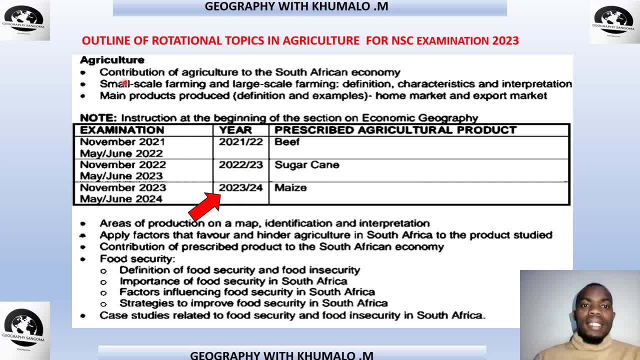 Each year. So now here we look at the contribution of agriculture to the South African economy. We are also going to look at small-scale farming and large-scale farming, looking at the definition and characteristics and how to interpret that Main products produced, definitions and examples, and then we are going to look at the home and export market, as I've said, 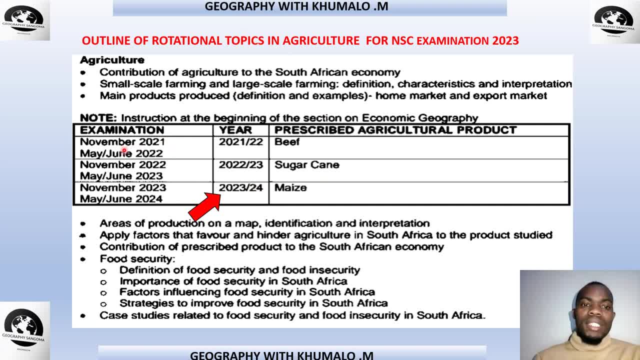 Now, if you look at this table that is in your exam guideline Grade 12, you see that we are not going to do beef agricultural products. we are not going to do beef because it's for 20. it was for 2021. we are not going to do sugar cane because it was for last year's group of grade 12. 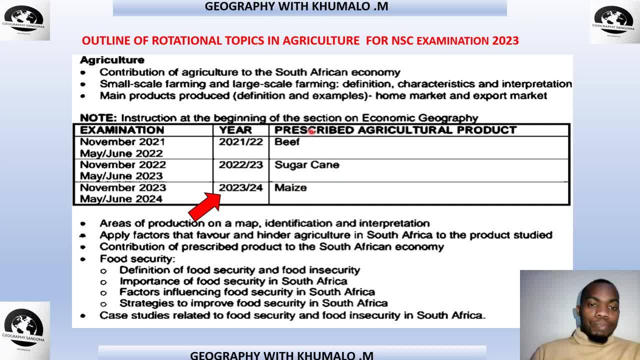 you are going to do maize, so you are going to do maize. that's why there is an error there. so that is one of the most important things that you should be aware of as you are studying across these agricultural topics- and there are some that i'm still going to- there are some that i'm still 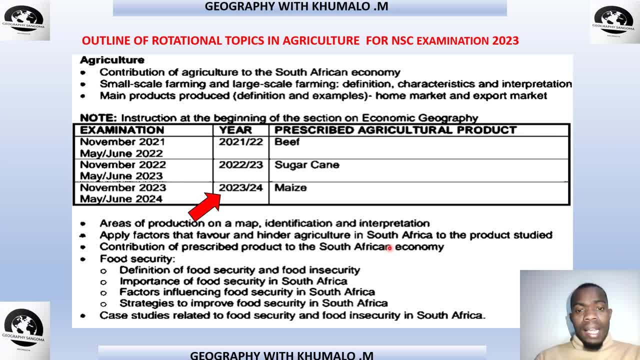 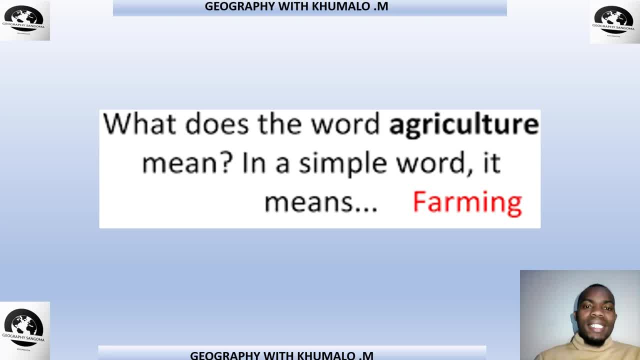 going to show you that are are prescribed for the year as we go to mining and other topics. now, what does the word agriculture mean? in simple way, it means farming. but now farming can be different. it can be livestock farming, it can be poultry farming, of chickens, it can be crop farming. 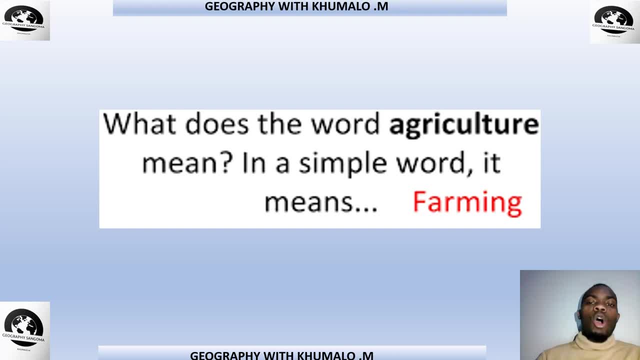 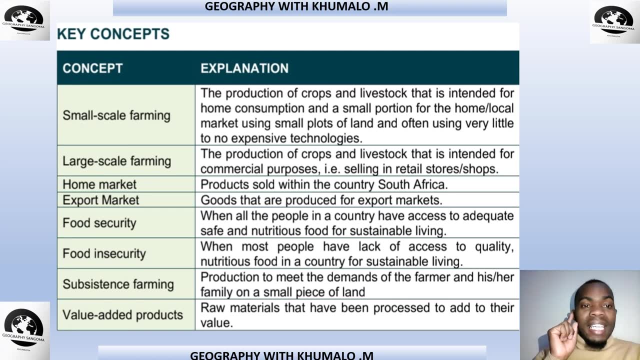 it can be family farming, it can be forest farming, it can be farm farming, it can be fruit farming. So the way that we use is farming or agriculture. So in simple terms, it's farming. Now I want us to look at the key concepts for this topic. The first one will be small scale farming, large scale farming, home market, export market, food security, food insecurity, subsistence farming and value added products. 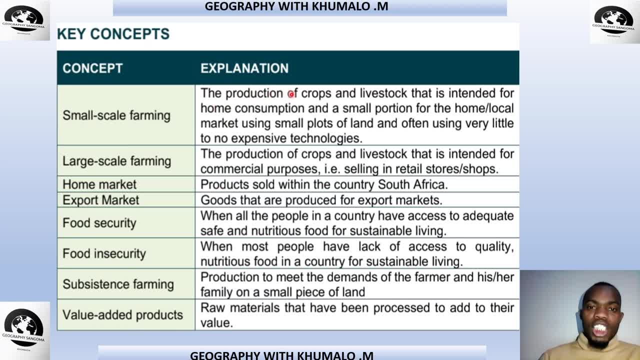 Now the small scale farming: the production of crops and livestock that is intended for home consumption, and a small portion for the for the home or local market, using small plots of land and often using very little to no expensive technology. So here we don't use, there are no much costs that are needed for this one. Then we've got a large scale farming: the production of crops and livestock that is intended for home consumption. 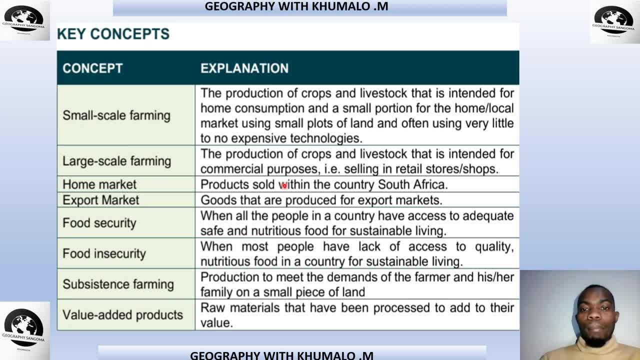 So here we don't use. there are no much costs that are needed for this one. Then we've got a large scale farming, the production of crops and livestock that is intended for commercial purposes, For example selling in retail stores and shops. Then we've got a concept of a home market, which is very important: grade 12 home markets, its products sold within the country, South Africa, as you're doing, the economy of South Africa. then we've got export market, goods that are produced for exports market which we are going to sell beyond South African borders. 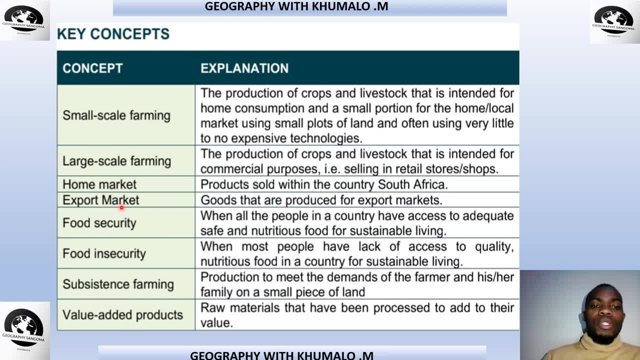 Now that these regards are fairly self有. In fact, we bring from rural Africa, from many countries, So we bring from rural Africa. Now, when we look at the industry, when we are talking about också food production- that we talked about earlier- and species safety, at the moment, the cause rather of Who is a madre media? Now the real point that we should mainly focus on is the buying from our country or overseas. now al jazz. Then we are going to get the concept of food security, Which is when all the people in a country have access to adequate, safe and nutritious food for sustainable living. the important 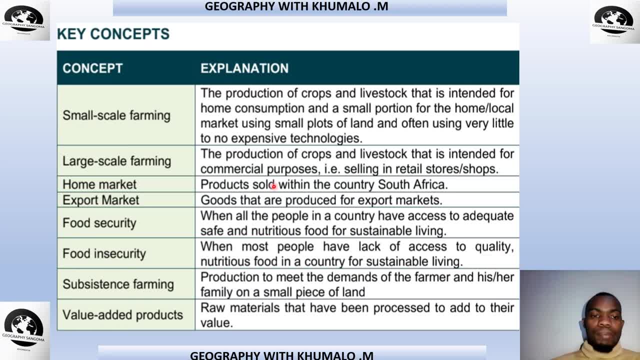 food in a country for a sustainable living. then we've got subsistence farming, which is production to meet the demands of the farmer and his family on a small piece of land. so this is the same as we say farming to feed your family. it's farming to feed yourself and your family. then we've got 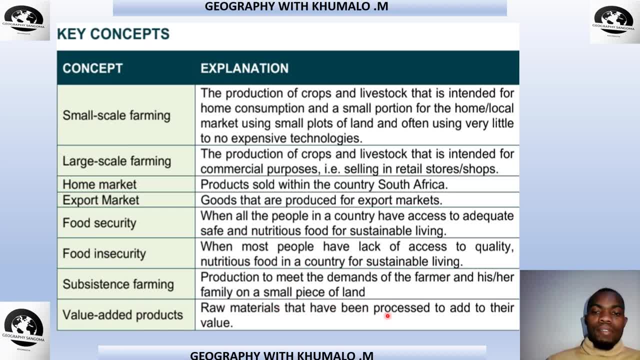 value-added products, now raw materials that have been processed to add to their value. so these are products that have been produced. we have talked about the value-added products in previous lessons because, uh, we talked about raw material changed to be processed- good, which we call them value-added products that we sell in the tertiary sector and get money. 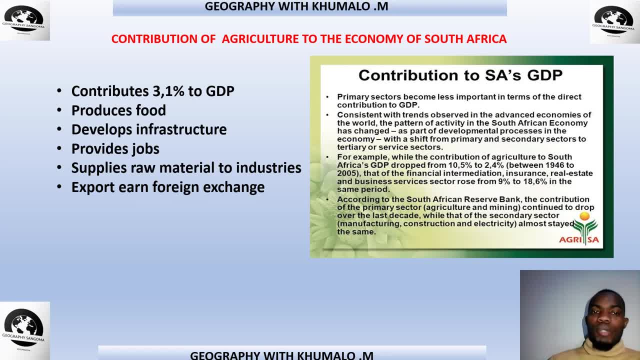 now, how does agriculture contribute to the economy of south africa? it contributes 3.1 percent to the gdp. remember this. we are working with figures, so they might increase, they might decrease. that is why here i've placed in a a small a text there from the agri. 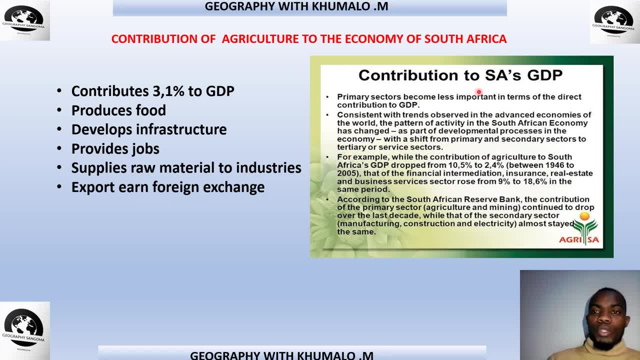 south africa. agree, south africa the contribution to south africa's gdp. so now it contributes to the gdp of south africa and how does it contribute to the gdp of south africa? it contributes 3.1 percent to that gdp. also, agriculture produces food, as we know that. 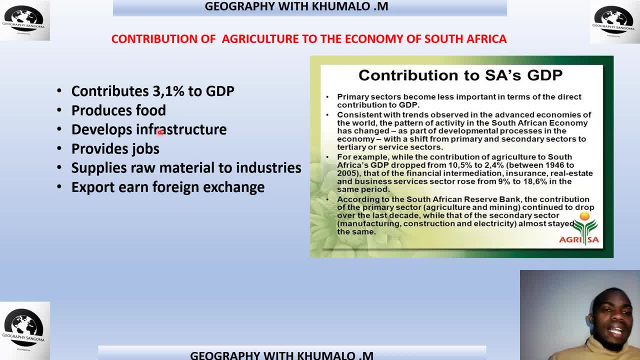 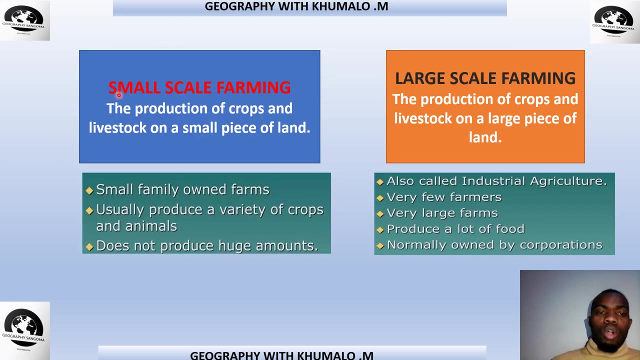 it deals with farming crops and livestock farming, develops infrastructure, it provides jobs, it supplies raw materials to industries and also these raw materials can be exported to earn foreign change. now I want us to also go back and look at small-scale farming and large-scale for me now I 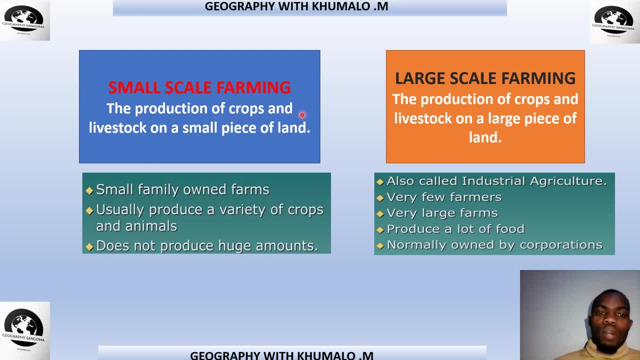 said, small-scale farming is the production of crops and livestock on a small piece of land. so, bear in mind, on a small piece of land, while the large-scale farming is production of crops and livestock on a large piece of land. now look at the characteristics now of a small-scale farm. 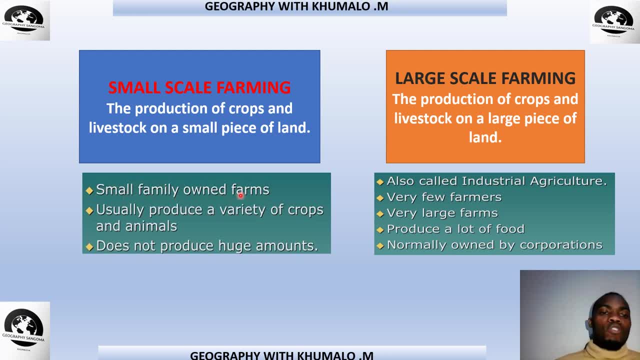 it's small, family owned farm, so this is owned by the family- usually produces a variety of crops, so it is a monoculture. that means they produce. it's not monoculture. I mean- sorry, forgive me for that- it's not monoculture that the farming different crops and animals they don't necessarily focus on. 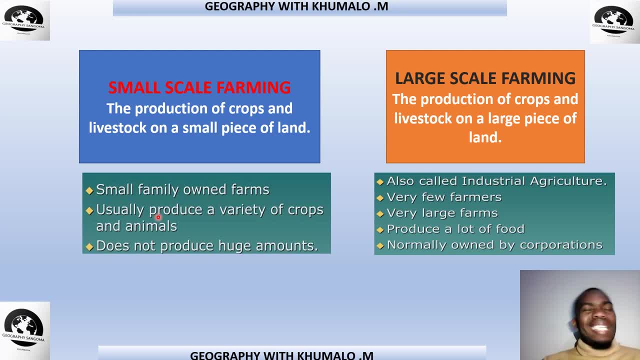 one and does not produce huge amount. so it can be a variety of crops that are planted but they don't produce a huge amount because, remember, they are not selling. it is small, family-owned farms. then now we come to large-scale farming. characteristics, also called the industrial agriculture. very few Farms, it has very few Farms, a very large Farms. it. 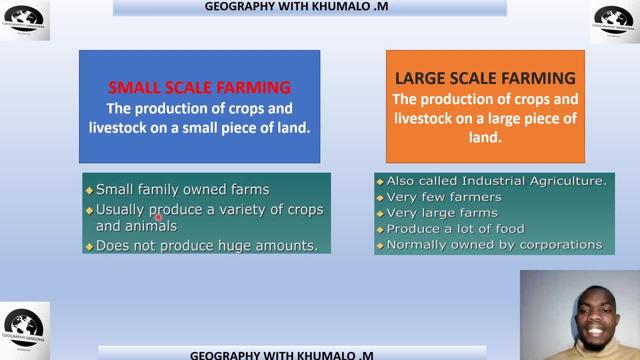 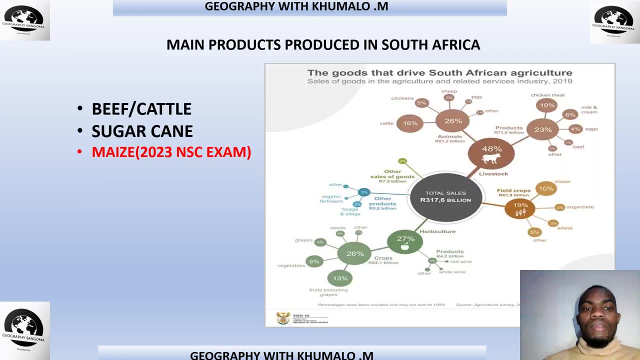 produces a lot of food and normally owned by Corporation, which is companies, agricultural companies, then the main products that are produced in South Africa with beef or kettles, sugar cane and maize, but for this year we are going to look at maize. remember, always remember, that when you are studying grade. 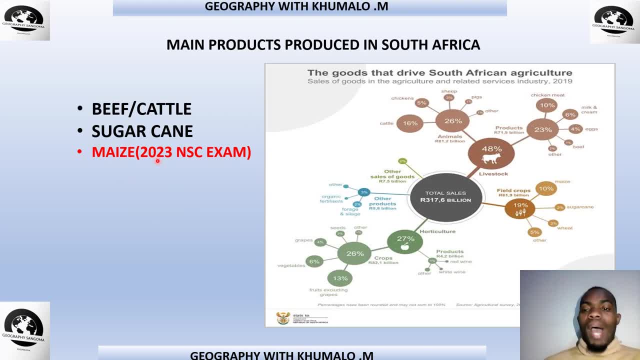 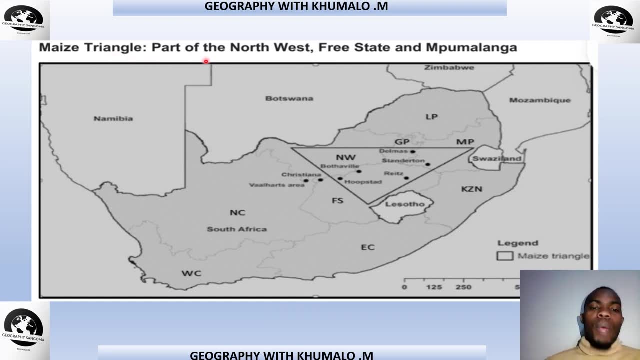 12 this year. we are looking at maize as our agricultural product for 2023.. now let's look at maize, the triangle of maize. where in South Africa do we find maize? parts of the Northwest province, the Free State and Malanga? so it's a triangle, three provinces, that we get. 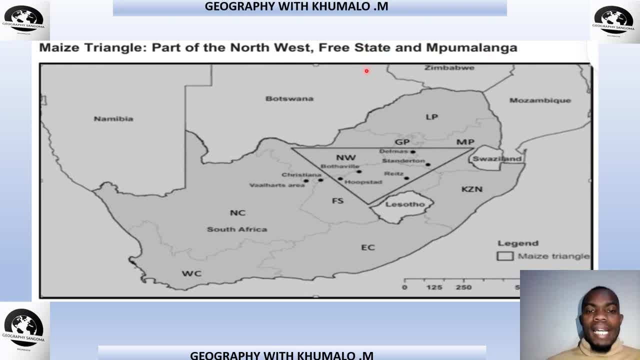 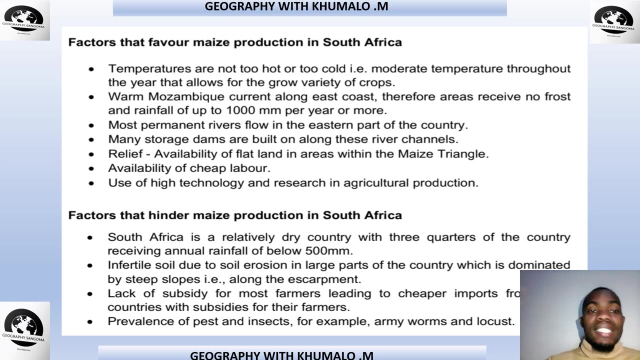 raised it will be Northwest Free State and malanga and salt. so you must know where in South Africa is this crop being farmed and then move to sectors that favor the maize production in South Africa. now, the factors that favor they're the same as fighters that it, other factors that 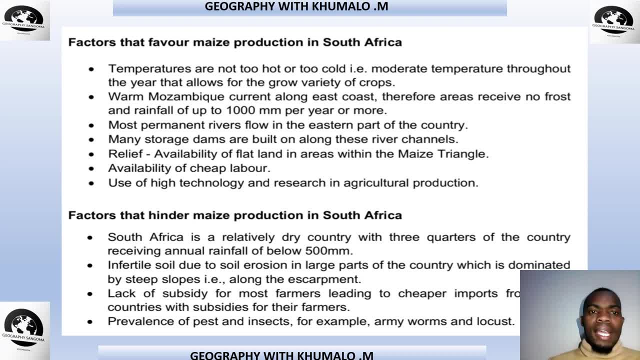 uh promote, or the vectors that a a a, those oppositions, factors that allow a good production of maize. so we're looking at temperatures that are not too hot or too cold, for example, moderate temperatures throughout the year. that allows for the grow of variety of crops. so our temperatures must not be too cold or too hot. 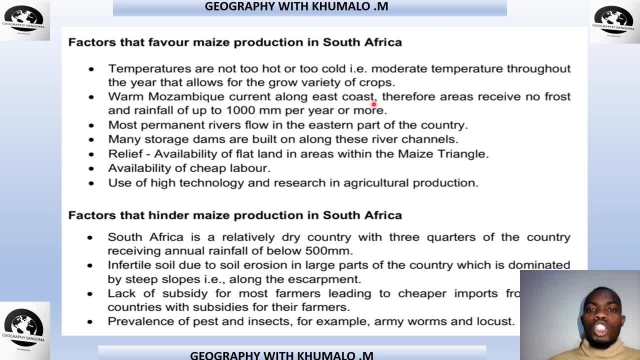 then warm was a big current along the east coast. therefore, areas receive no frost and rain up to 1000 millimeters per year or more. so we need frost free areas. so the the the other factor is that we need a frost free areas and an area that experience rainfall of about thousand. 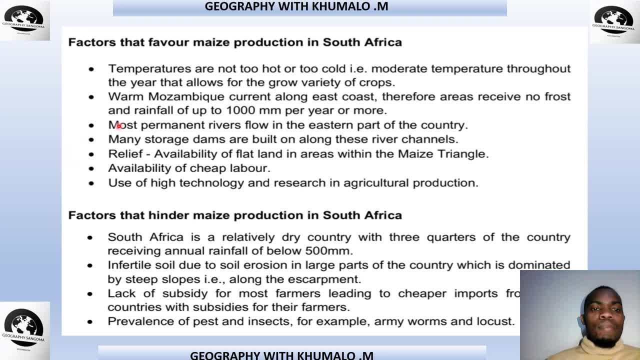 millimeters per year or more, then most permanent rivers flow in the eastern part of the country. so also we need a permanent rivers which ensures that there is a constant supply of water for the crop. many storage dams are built on along these river channels. they relieve availability of flat land in areas within the 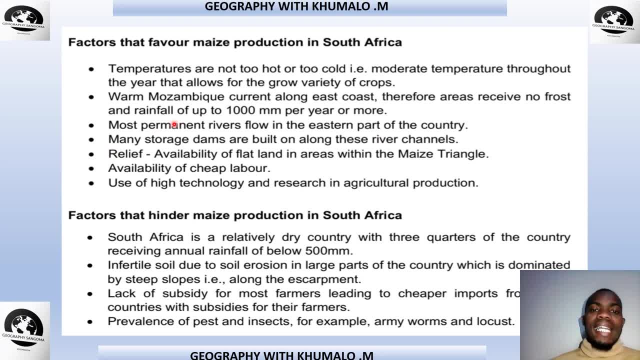 main triangle, so we need a flat land to plant this type of crop. and then availability of cheap labor. yes, you know cheap labor. they will take people who are staying in those areas to to pay them as to offer them jobs in that area. so they must be availability of cheap labor. 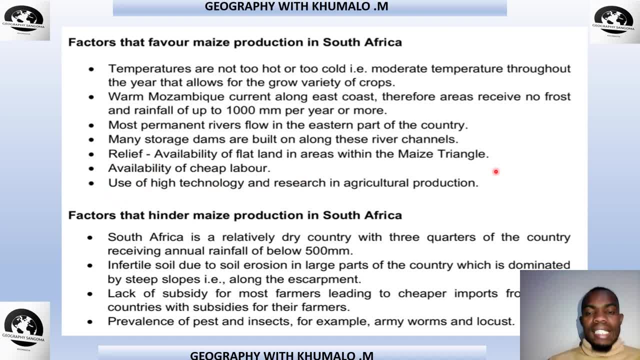 use of high technology and research in agricultural production. this includes the quaternary sector now, because it has to do with high technology and research in agriculture. so they have to continuously research, research on how can they meet the demands of the people in the home market and in the export market, how they can keep the demand- uh uh, the sub, so that they can. 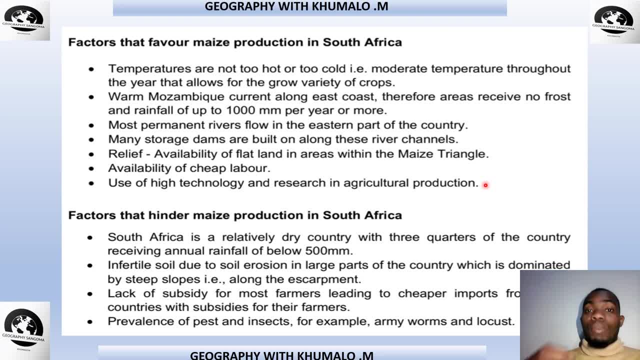 supply, uh, to keep up with the demand. so when they supply, that is when they produce more and supply and ensure that all their customers they have or they get the product, and then when the demand becomes high- grade 12- obviously the supply must be high. you can't have a demand that is high in this. 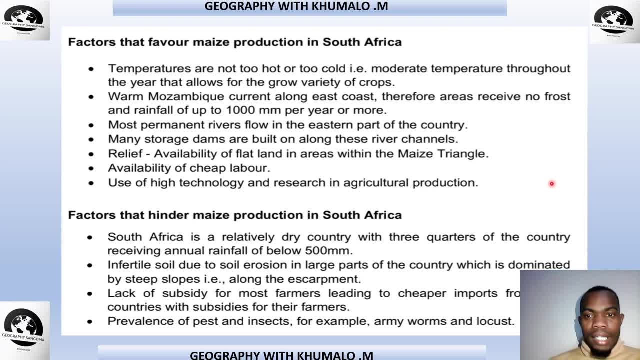 then you will be not working at a profit. then we are going to look at the factors that hinder, which are negative factors. they hinder maize production in south africa. south africa is relatively dry country, with three quarters of the country receiving annual rainfall below 500 millimeters. you see, so we said here we wanted thousand millimeters of rain per year, but south 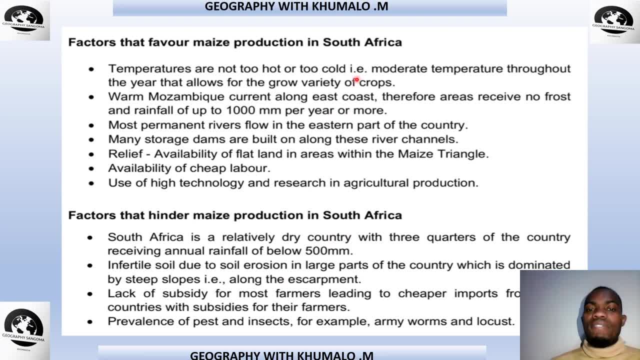 africa receives below, even below half of the rain that is needed there. so that is a negative factor about south africa- in the industry of maize production and then in fetal soil due to soil erosion in large parts of the country, which is dominated by steep slopes. remember we said we. 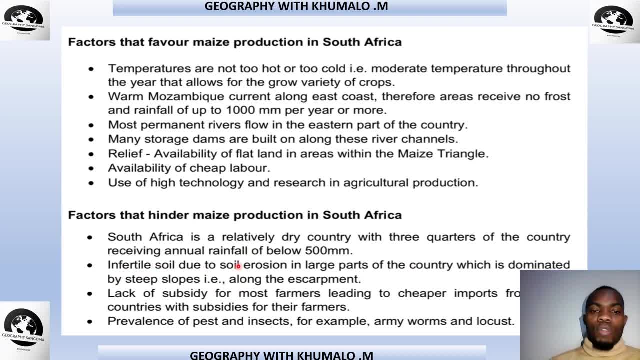 want flat land. but now here we in south africa, we've got a dominated uh land forms of steep slopes along the escapement, the lack of subsidies for most farmers, leading to cheaper imports from other countries with subsidies for their farmers. so a subsidy it's a sub it's a. 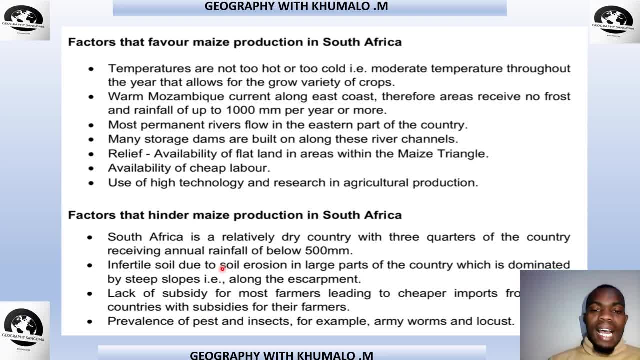 support fund. so this is the funds that are given to to farmers so that they can maintain their farms. and then we also look at the prevalence of pest in insects. remember, we've got arm of worms and locusts that come and feed on the crop, which process. 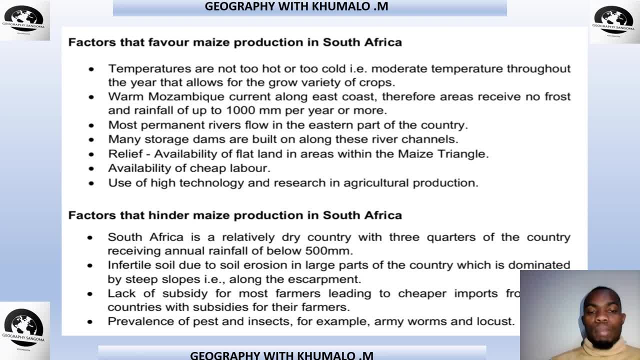 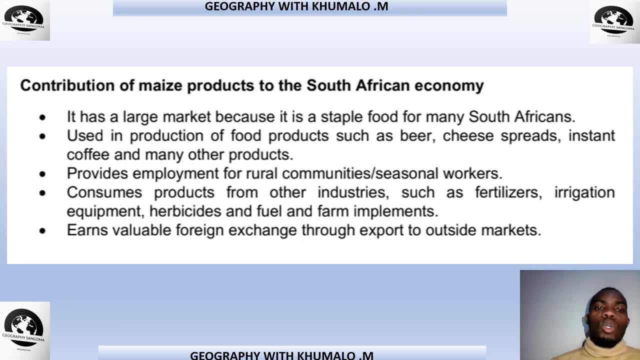 which poses a negative threat in our maize production. then grade 12s we are going to move on here and then ask ourselves how maize contributes to the south african economy. now, maize it has a large market because it is a temple food terms isn't korean south africas. so most of us we use maize, we we get. we use maize in different 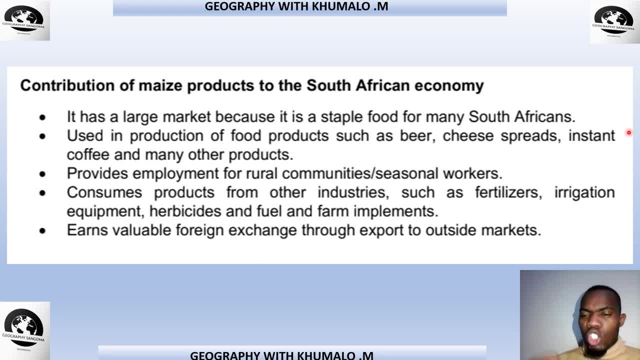 in different types of food, like cooking your pub, a lot of things that can be done with maize. so now it has a large a market because we south africans we use too much maize. imagine you always eat pop at home, how many times you eat pop and how many. donne möglich en Creative su shape loores surfaces se sacrilegio de pap. 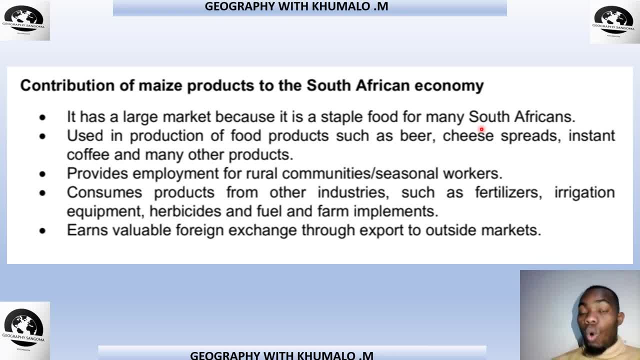 many kgs of maize meal do you buy at home? so you can see that we use a maze more and more here in south africa and it is used in the production of food products such as beer. yes, we use. someone will ask: how do we use maize in beer? yes, in the process of making beer they use maize cheese. 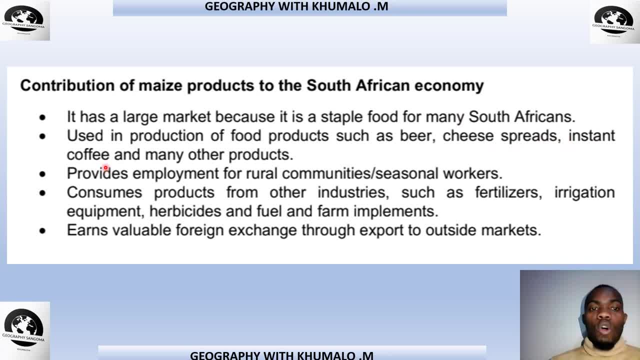 spreads we. they use also maize instant coffee and many other products that we can use maize to produce, and then now maize products also provides employment for rural communities and seasonal workers. now, seasonal workers will be those workers who work at a certain period of time where there is a time to cultivate land. 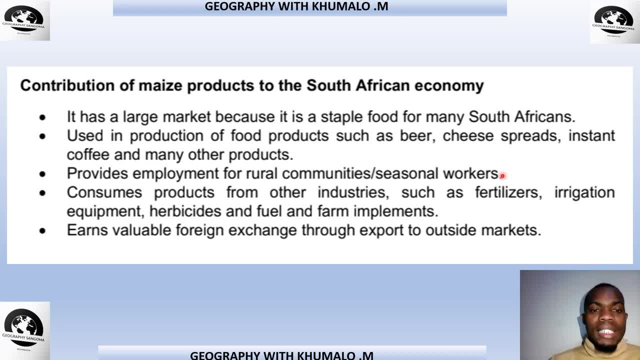 and farm maize, and also when it's time for yielding, so it provides employment. so that's also how it helps the economy. now we also look at it consumes products from other industries, such as fertilizers, irrigation equipment and herbicides, and fuel and farm implements, so it 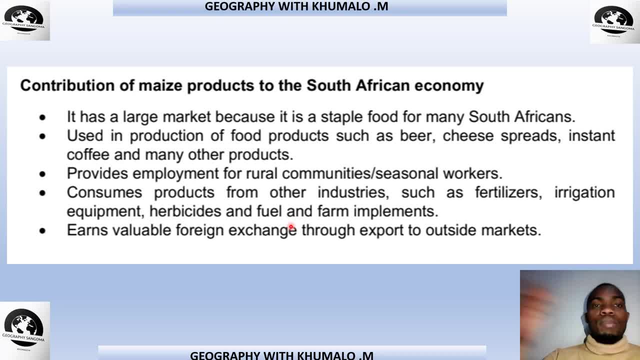 consumed products. so now some of the products from different secondary factories, they are going to come here and they are going to to be used to to get rid of things like of animals, like the insects, like the pesticides, the the insects, sorry to produce things like pesticides to deal with insects so that we can protect our plants from those. 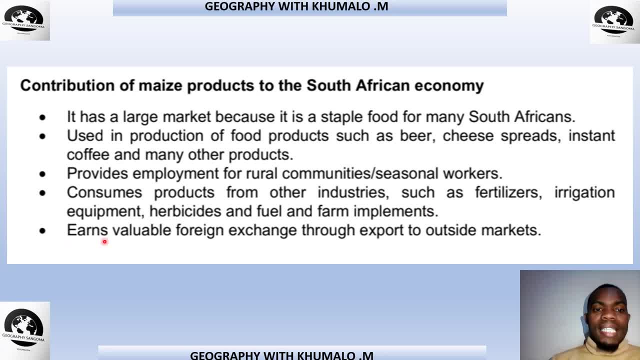 insects, and then it ends as a valuable exchange through exports, as we export them outside the market. now, as you can see, grade 12- it's very important to understand here that the main word today is economy. so all these factors must lead to the economy. you can see here: 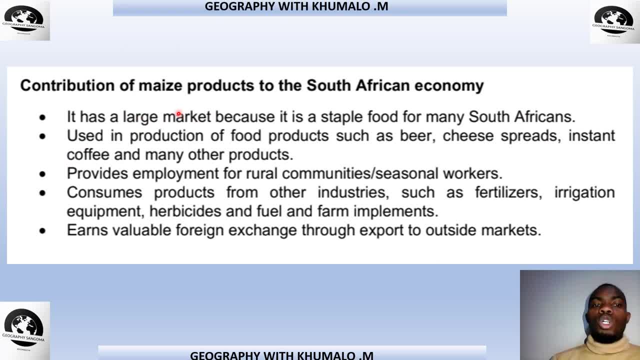 it talks about large markets. it's part of the economy. we use the production for food production. it's part of the economy. provides employment. it's part of the economy. and then it consumes products and industries. it's part of what the economy. and then we also look at foreign exchange, export and market it. 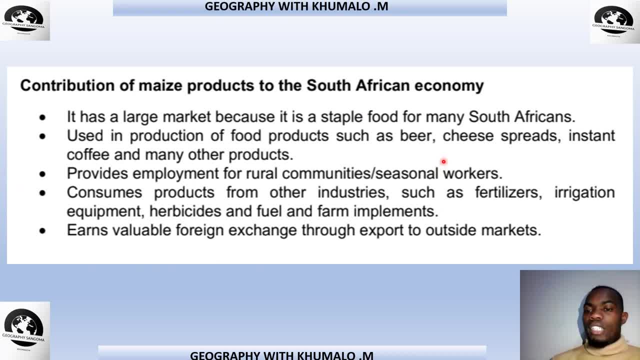 shows that all your factors, they are related to the economy. so you must be aware, when you are dealing with these contributions and they ask you how it contributes to the economy, to stick to the economic factors, not, um, environmental factors or whatsoever, but stick to economic factors. and 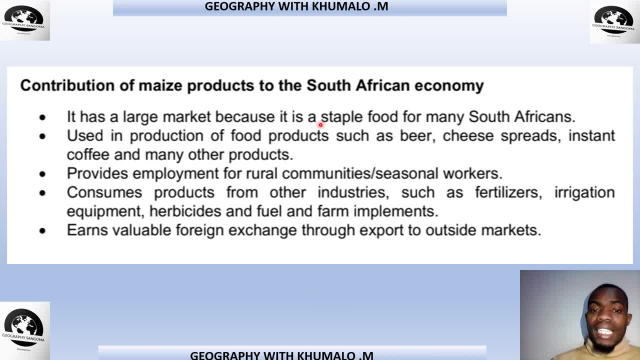 now you must always pay attention, because an exam question can ask you that they want those that are in the extract or in the case study, or in the in the infographics. then you have to check, uh, which one of these is there on the picture? don't name the one that is not there on the picture. and then 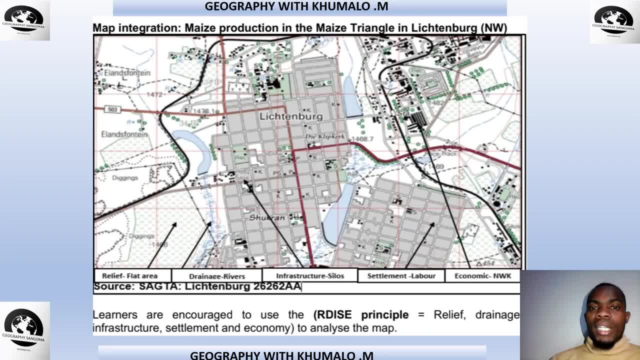 that will bring us now on how. now question three can be asked. remember that you have a question three which is map work on your paper. two now: how to integrate maize production in the maize triangle in lindenberg on north west. now you can see, you must be able to see, that there is flat relief there. 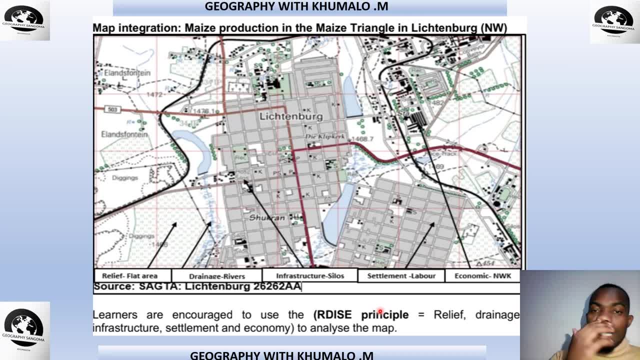 the drainage of rivers. and then, but now here the important part, grade 12 will be. you must be able to use the r d i s e, which is the relief, which is flat area. you can see that there is flat area there. drainage of a river: you can. 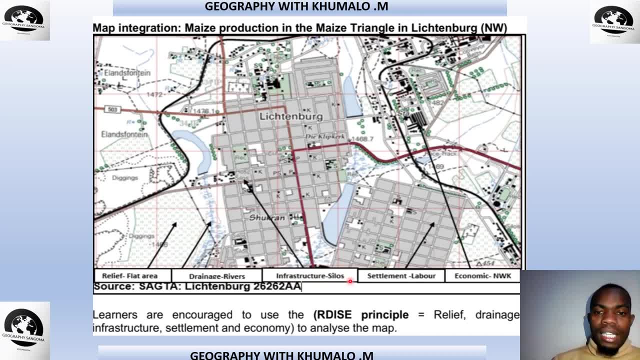 see the drainage of rivers, the infrastructure, the infrastructure, the settlement labor, that they are people who are snakes to labor force there and there is an economic uh network there there is an economic network and in form of industries. so you look at all these uh five factors, uh, in order to 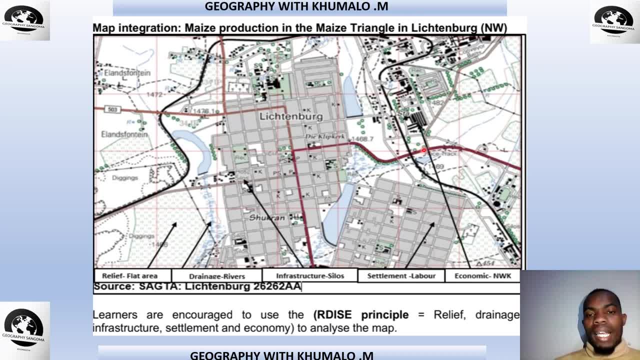 determine or to interpret the map. a, a, a question in terms of the maze triangle. and now, uh, that is very, very important for questions three. now i would like you to go back and listen, rewind this video, go to your, your youtube, watch this video, like, subscribe and share with all your classmates. this is all from me. kumalo m the. 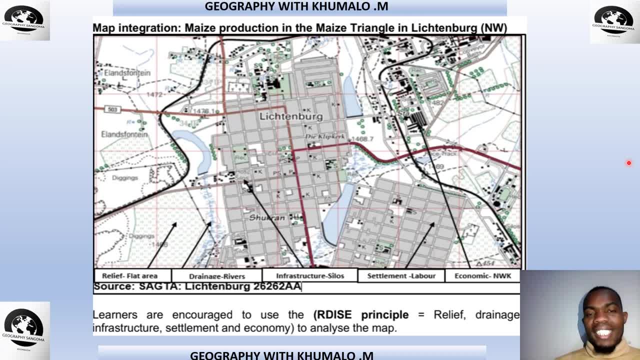 geography sangoma. have a lovely day and don't forget solve as many previous question papers after listening to this lesson.